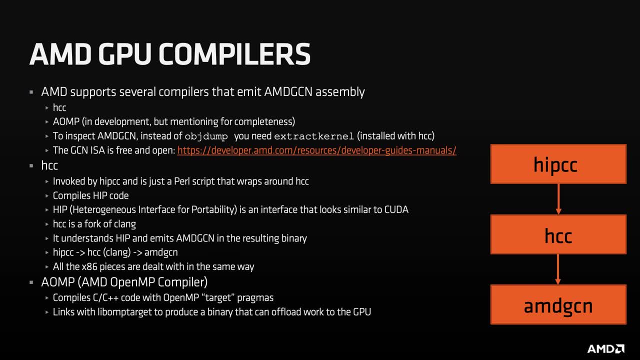 a fork of Clang. So any options, flags that you're familiar with from Clang will work with HCC, With HIPCC, and HIPCC will pass them down to HCC. The compiler will emit AMD GCN assembly that runs on our devices And we'll also do a second pass, as Noel has already mentioned. 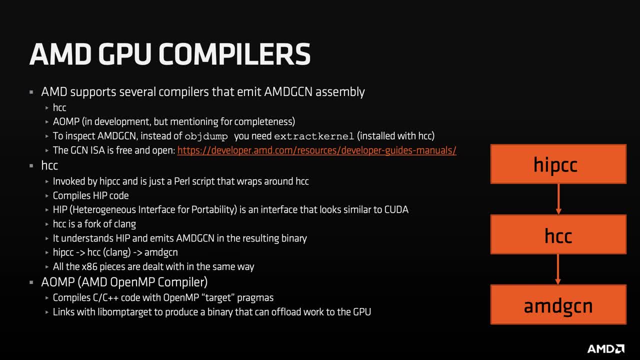 to compile all the x86 pieces for the host. So it's worth mentioning here that once you have compiled HIP code you get essentially an executable that can run on the device. You may wish to inspect the assembly that runs on the device and you can do that with. 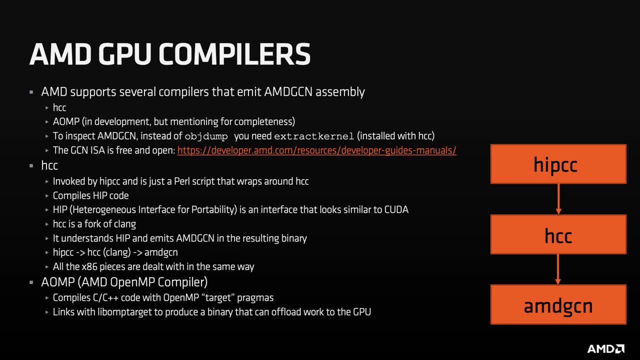 a piece of software we provide as part of Rockham called extract kernel, And if you do that it will output a text file containing all of the AMD GCN And you can do that for a pretty large amount of time. the command is a little bit tricky. Usually, once you've compiled HIP code you get essentially 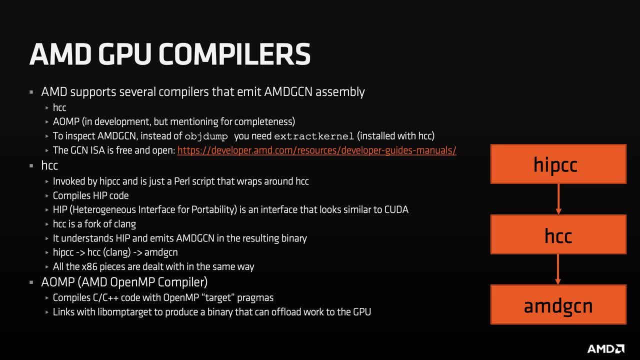 a executable that can run on the device. you may wish to inspect the assembly that runs on the device And you can do that with a piece of software we provide as part of Rockham AMD GCN instructions that run on our devices. You can think of it as the AMD GCN equivalent. 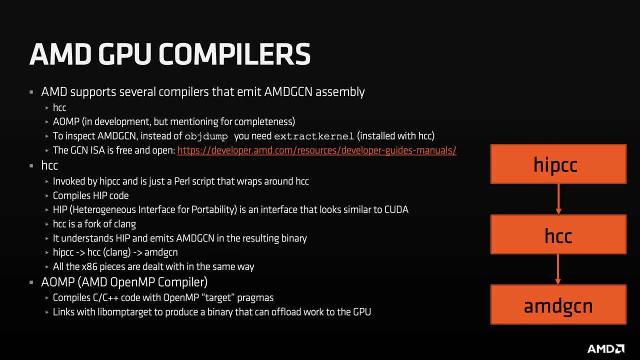 of OBJ dump for dumping x86 assembly on the host, if you've ever used that. It's also worth noting that our instruction set architecture is completely free and open source. I've provided a link here to resources where you can go and read about what our instructions do. It might. 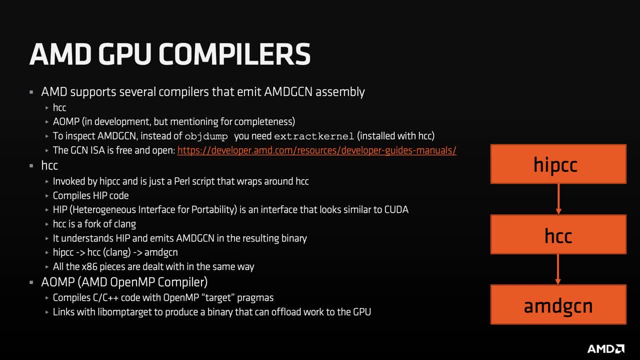 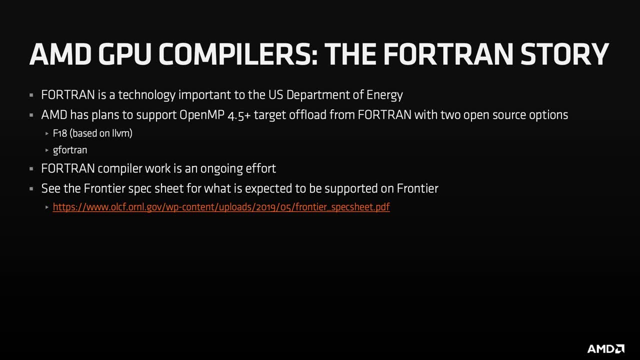 be interesting to some of the people that like to delve deep into the weeds. Okay, so Fortran. We realize Fortran is a critical technology to the Department of Energy. It's very important that Fortran is supported. AMD has plans to support OpenMP 4.5 and beyond target offload pragmas from Fortran with two. 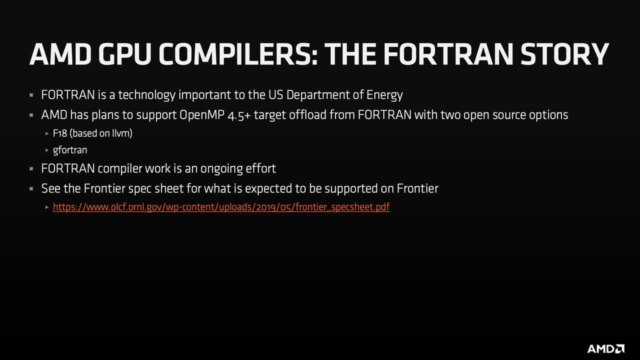 open source compilers. You can use GFortran or you can use a compiler called F18, which is based on LLVM. There's a very active development community working on F18, and I encourage you to provide feedback and interact with them if you're interested. 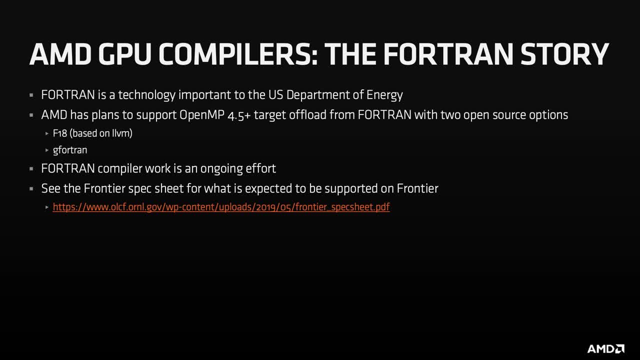 But in general, Fortran compiler work is an ongoing effort and I encourage you to look at the Frontier spec sheet if you're interested to see what will be supported on the Frontier system, and you can go to this link and see what will and will not be supported. That's all I have to say. 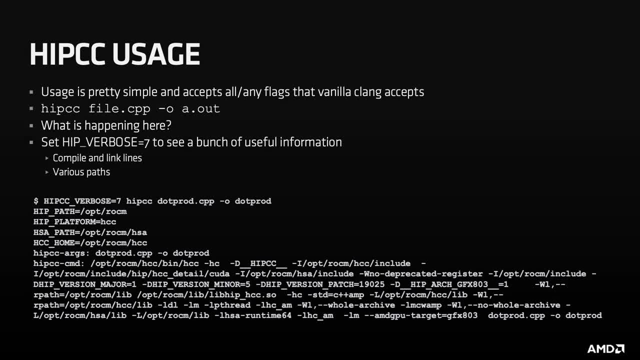 about Fortran. So how do I use HIPCC? So, as I mentioned earlier, the usage is pretty simple. It accepts any client flags since HCC. So if you're interested in using HIPCC, you can use HIPCC. 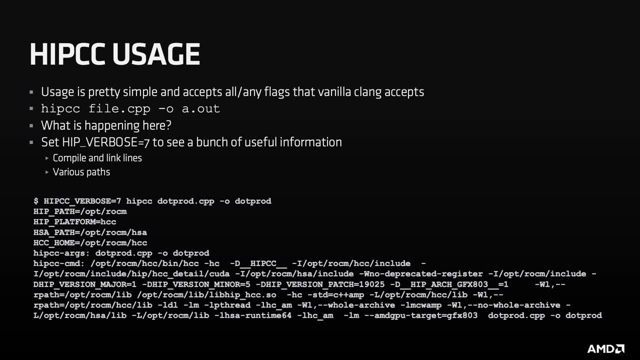 There's a Clang fork. So here I have an example where I'm compiling a file called filecpp and producing a binary. So you might ask the question: well, what's happening here? You can set the environment variable HIP underscore- verbose equals 7, to see a bunch of useful information like: 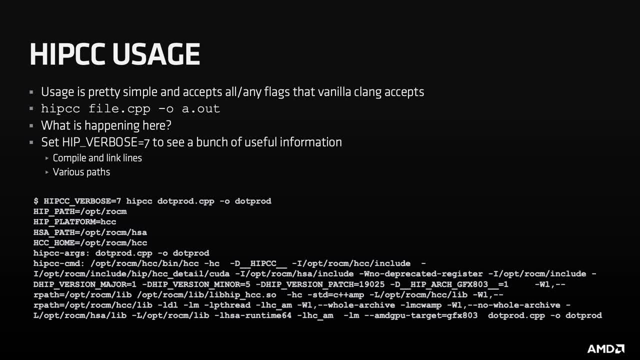 compile and link, compile lines and link lines and various paths to runtime libraries and other things that you might find interesting. So here I have example output from that. I've compiled a simple dot product application. You can see where my HIP install is located. You can. 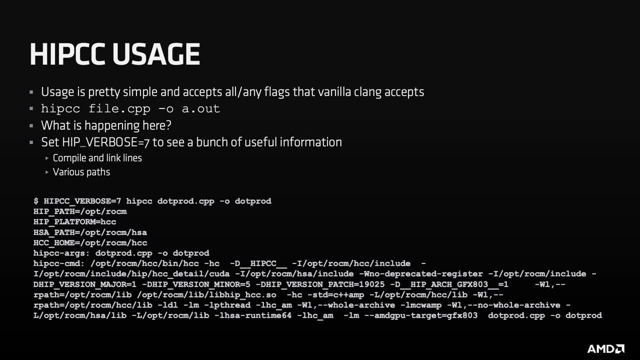 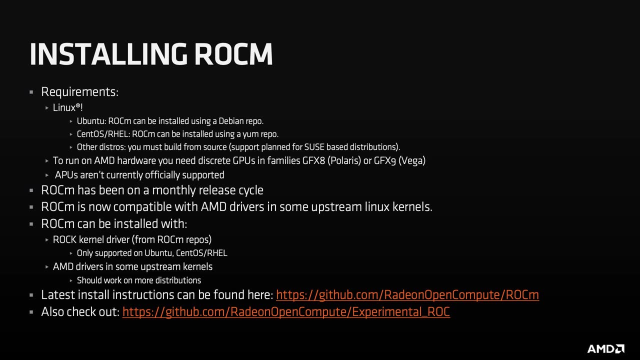 see that HIPCC is managing things like defines for what version of HIP I have installed, what architecture I'm running on that kind of stuff. Okay, To get HIPCC and HIP and all of the stuff that we've been talking about, you need to install something called Rockham And Rockham. 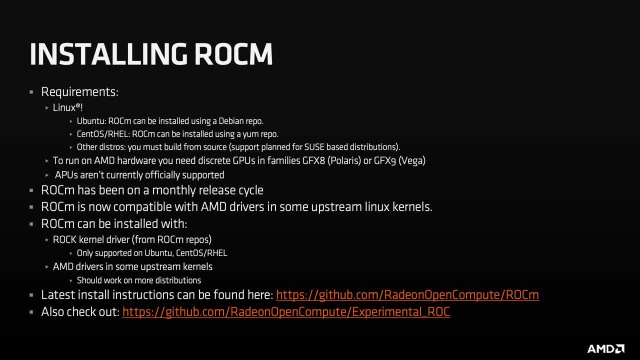 provides a lot of information, So you need to install something called Rockham, and Rockham provides a lot of information, So you need to install something called Rockham, and Rockham has several requirements. The first requirement is: you must be on a Linux-based system. We support. 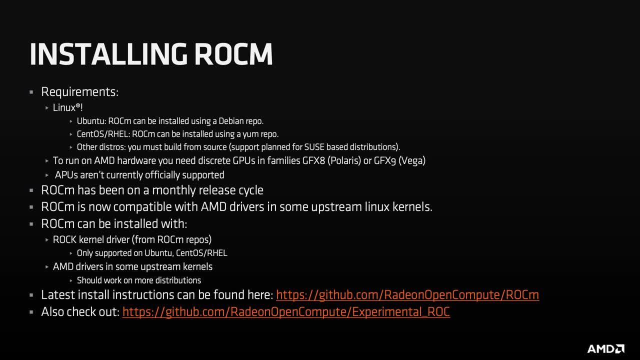 Ubuntu CentOS slash RHEL You can install from your system package manager by simply updating your sources to include the Radeon repository. For other distributions you probably have to build this from source And we have support planned for SUSE-based distributions in the future. 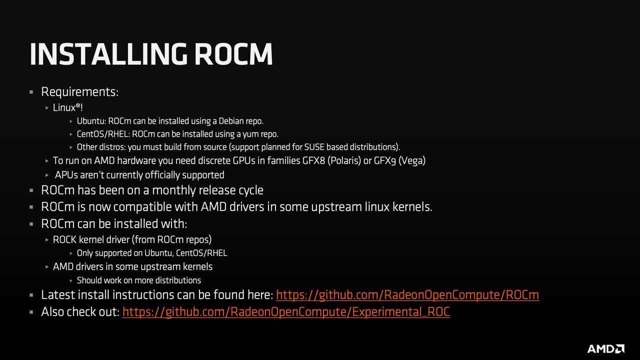 To run AMD hardware you obviously need an AMD device. We'll support Graphics 8 and Graphics 9 devices, So that's Polaris and Vega. APUs are not currently supported, So we're only supporting discrete GPUs. Rockham has been on a monthly release cycle. I think the most recent version is 2.4. 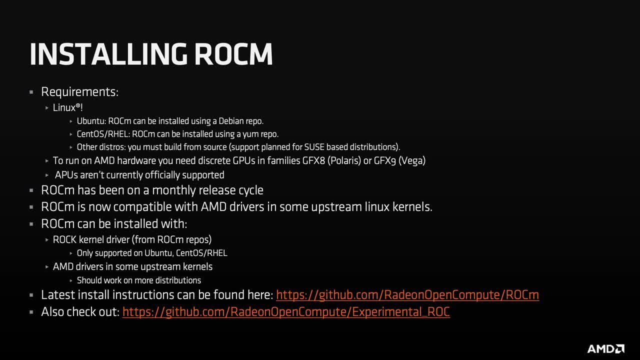 And Rockham is now compatible with the HIP app So you can install it on your system package manager with AMD drivers and upstream Linux kernels. So that's where we contribute essentially in the mainline kernel, our devices directly, as opposed to installing a kernel module, for example. Rockham can be. 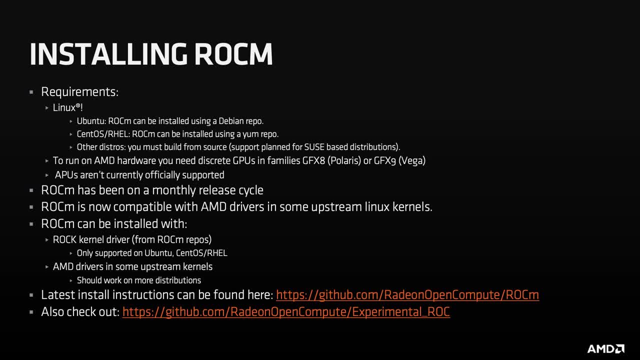 installed with the Rock kernel driver, which is simply a kernel module, And this method of installation is only supported under Ubuntu or CentOS, And for the other versions of whatever distribution you're using, you'll need to use the upstream kernel- Upstream Linux kernel. I've also included links to installation instructions here, which you can look at in. 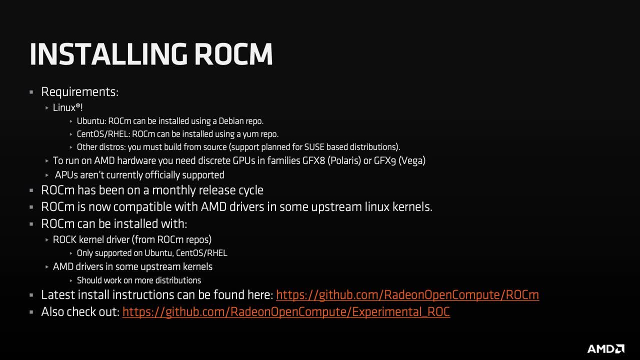 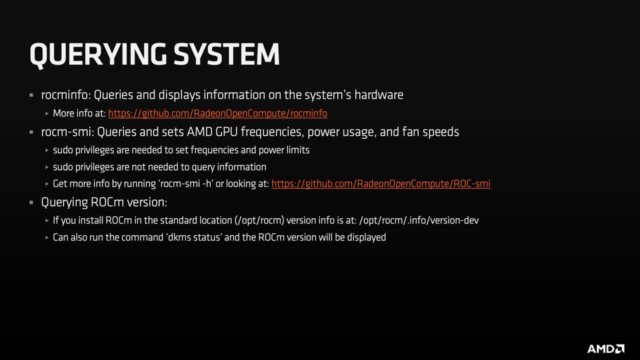 your own time. Okay, So once you've installed Rockham, how do you know that you have installed it correctly? We provide a piece of software called Rockham Info, which will display information about all the HSA-compliant devices on your system, like AMD CPUs and AMD GPUs. 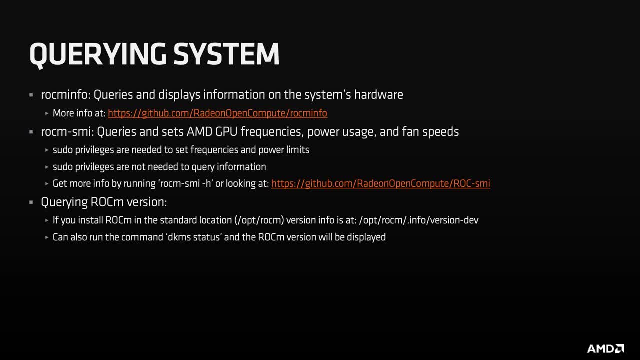 Another binary we provide is Rockham-SMI, which lets you, for example, set and monitor frequencies, monitor power usage, set fan speed, things like that, And you'll need the requisite privileges to do things like set frequencies and you may not need. 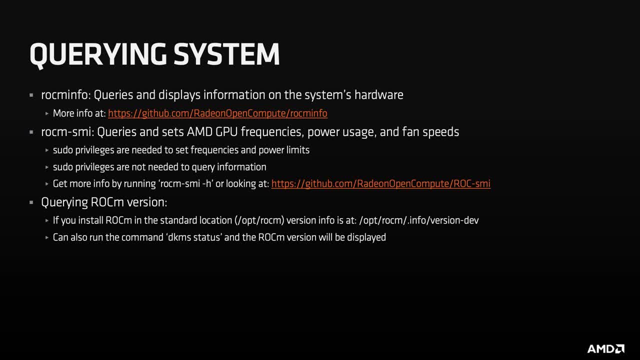 those privileges to, for example, just monitor them. You can also pass the dash H flag if you want to see all the available options you can pass to Rockham-SMI. If you install Rockham in the standard location, which is slash opt, slash Rockham, you can look at what version you have installed in. 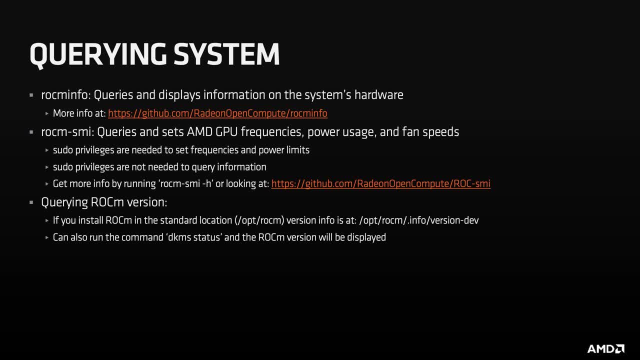 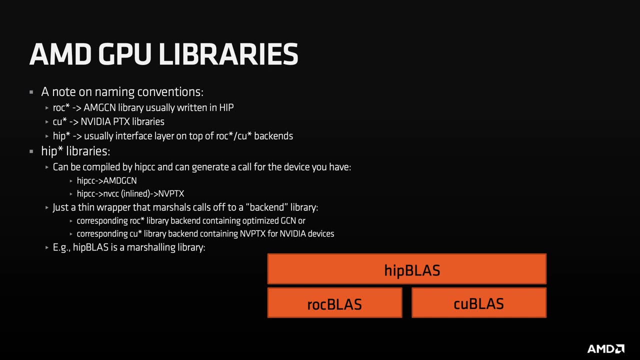 slash opt, slash Rockham, slash dot info, slash version dev, or you can use at list whatever you're comfortable doing. I think that's all I have to say there. Moving on to libraries, you might have realized there are a lot of Rock. 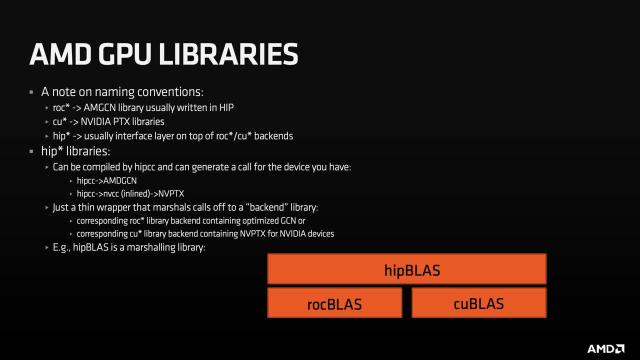 HIP and CU names. So I'd like to just clarify what we're referring to when we say these things. So anything beginning with Rock is an AMD GCN library. that's usually written in HIP. Anything that starts with CU is an Nvidia library And anything that starts with HIP is. 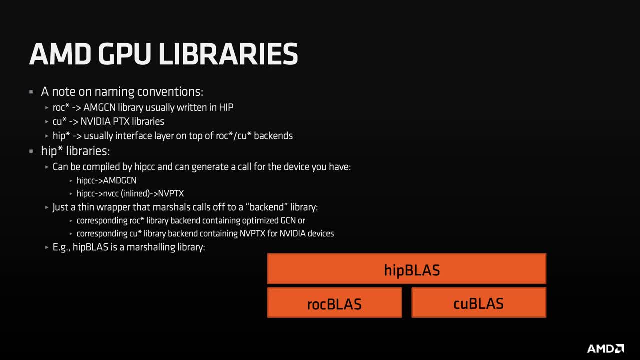 usually an interface layer on top of either the Rock or CU backends. So, for example, HIP BLAS is an interface layer between ROC BLAS and KU BLAS And if you have an NVIDIA device, KU BLAS will get called. 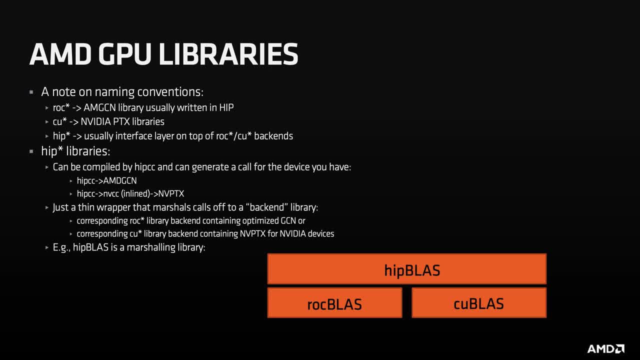 And if you have an AMD device, then ROC BLAS will get called. HIP. libraries can be compiled by HIPCC and they generate a call for the correct device, And the HIP layer is simply just a thin wrapper that marshals calls to the correct thing. 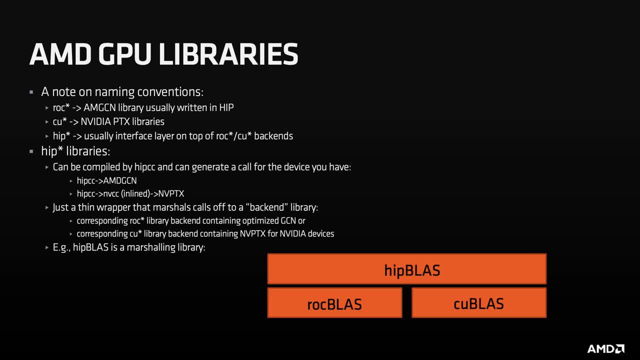 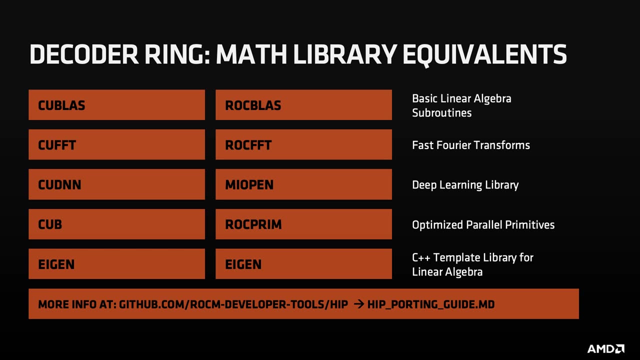 And we will replace the HIP call and inline a KU BLAS call, so there will be no overhead for running on NVIDIA devices. So hopefully this picture makes it clear what we mean when we say HIP versus ROC versus KU. This slide is basically just. 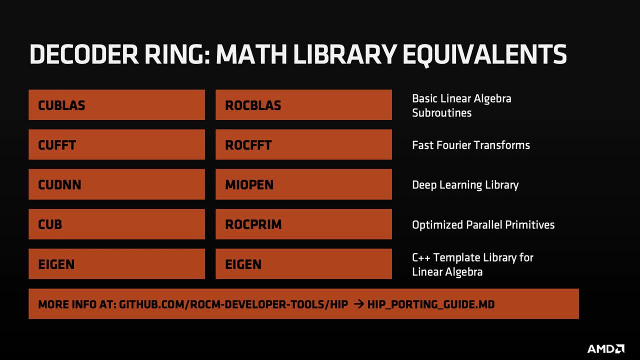 A Rosetta Stone that you can refer to if you're familiar with CUDA, and then you would like to know what the equivalent AMD library is for AMD supported devices, and I have that here for you to refer to later. If you want to install, for example, ROC BLAS, you can do a sudo apt: install ROC BLAS. 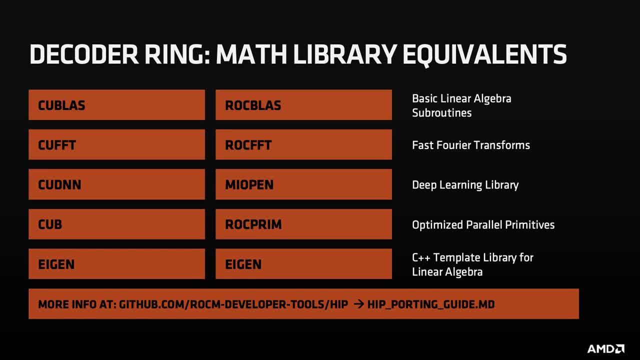 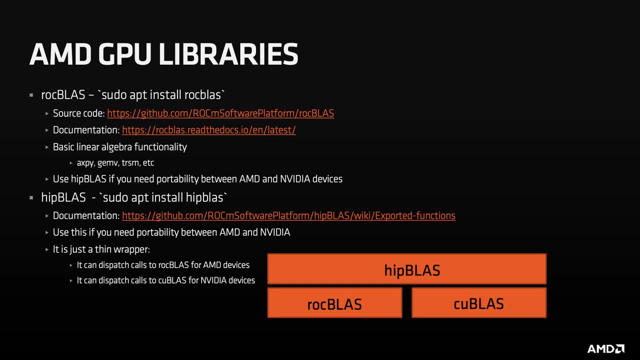 And here I have, for example, a point of the source code. It's worth noting that our libraries are open source and you are free to download them, contribute to them, report issues, fix issues. I've also included a link to our documentation. 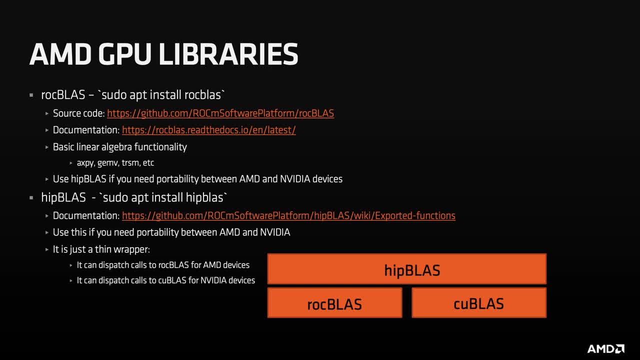 And just a note on ROC BLAS. ROC BLAS provides some basic linear algebra functionality: AXP, like level one calls, GenV like level two calls and TRSM like level three calls And you should use. You might ask the question: should I use HIP BLAS or should I use ROC BLAS? 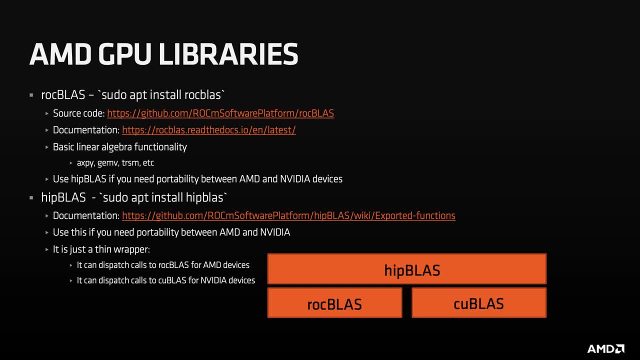 Well, if you want the portability, if you want to write one piece of source code and have it run anywhere on an AMD device, AMD device or an NVIDIA device, you should use HIP BLAS and let our compiler manage what gets called at runtime.